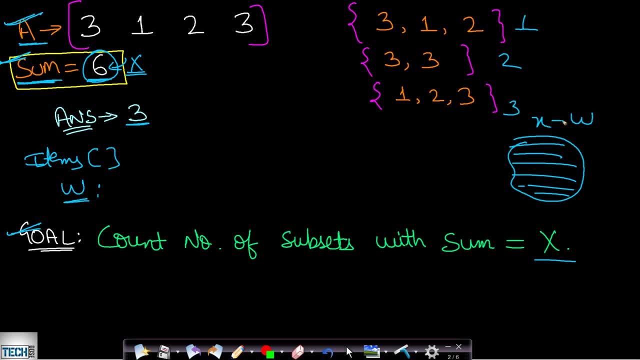 which you have filled. let's say you have filled x amount. x should be equals to w, It should not be less than w and it should not be greater than w. So this is a constraint, and our items is nothing but this array a. Now, these two inputs are both the same and you can also see that if you are. 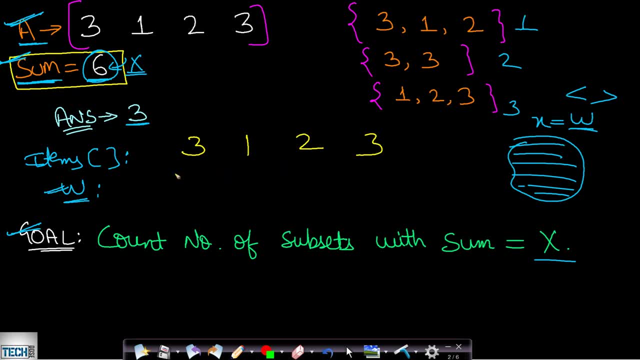 having this array- 3, 1, 2, 3- then you can form items using two possibilities. That means, for each item you will have two choices, just like in a 0: 1 knapsack, You can either include a 0: 1 knapsack or you can include a 0: 1 knapsack. 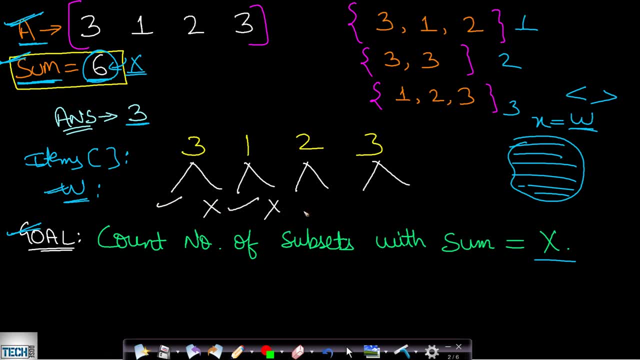 an item or you can exclude it. You can include an item or exclude it, and so on. So in this manner you can form all possible subsets and you can find the sum of all those subsets and see if it is equals to the given sum. If it is equals to the given sum, then you can keep a counter which will be initialized to 0 and 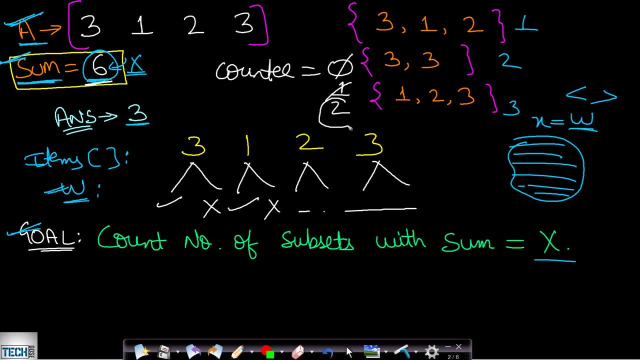 then you can keep incrementing the count values and whatever the count value comes at last, after seeing all the subsets, that will be our answer. This is a very simple approach for solving this problem. Now let us see the similarity of this problem with the subset sum problem. Now in the 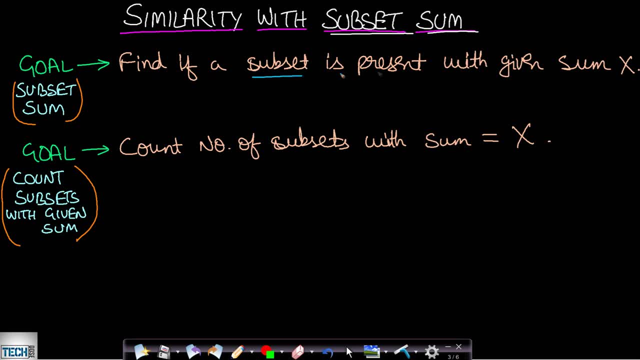 subset sum problem. our goal was find if a subset is present with the given sum x. There we needed to return true. if there was a subset in the given set so that the sum was equals to x, Then we will return true. otherwise we will return false. In this problem, our goal is to count the number of 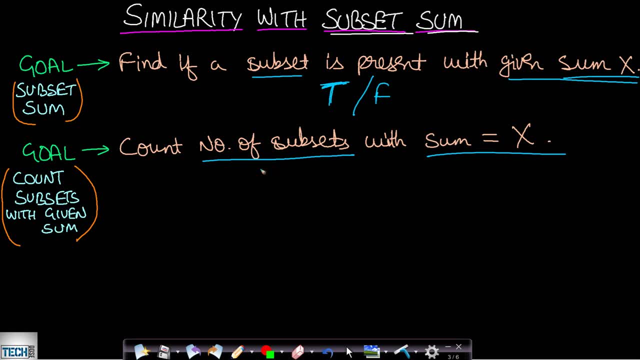 subsets with some value equals to x. Okay, So here we are actually counting. Therefore, the return type in the subset sum problem will be a boolean type, whereas in this problem it will be of integer type, since we are returning the count of the number of subsets. 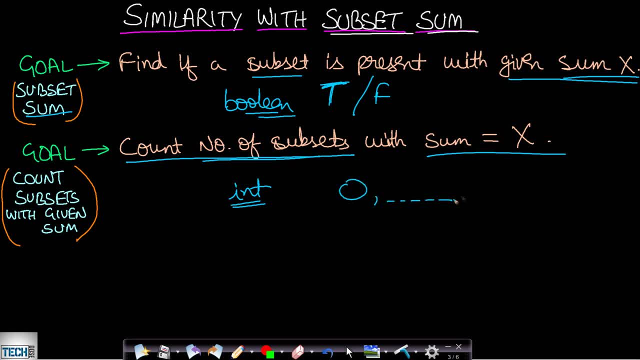 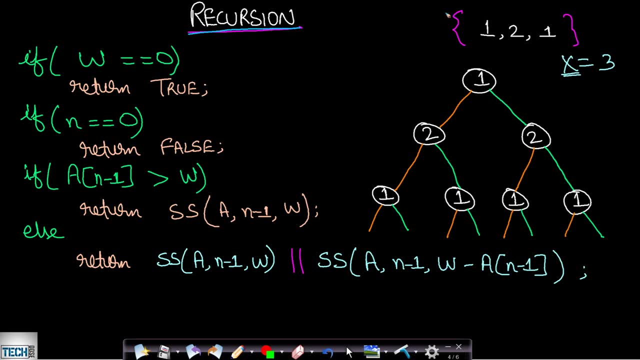 So the possible values here can be from 0 and it can go to any number. Okay, Now you can solve it very simply by using a simple recursion. So let us say our input is given here. This is array a and this is the given sum value x, which is equals to 3.. Now, if we draw a simple recursion, 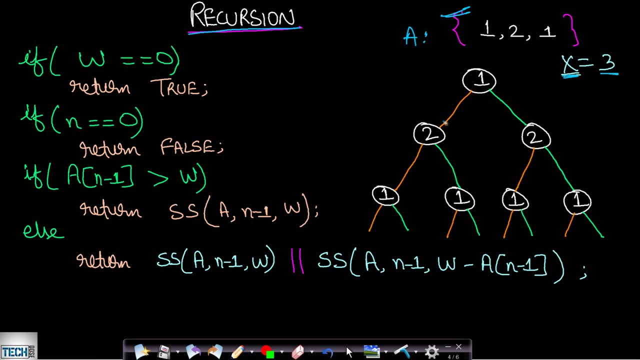 that is a tree diagram. then the red lines will indicate that the parent node will not be included and the green line will indicate that the parent node is included. So if you do not include one, you go to two. you do not include two, you go to one. you again do not include one. then what? 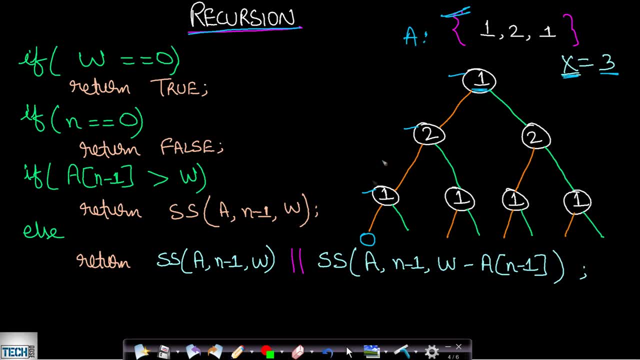 will be the sum value. Sum value here will be zero because we have not included anything. Now, if you include this one, then some value will come out to be one. You keep comparing with the given sum value, which is x. You also keep a counter here. Okay, So count can be equals to zero. Now you will backtrack. 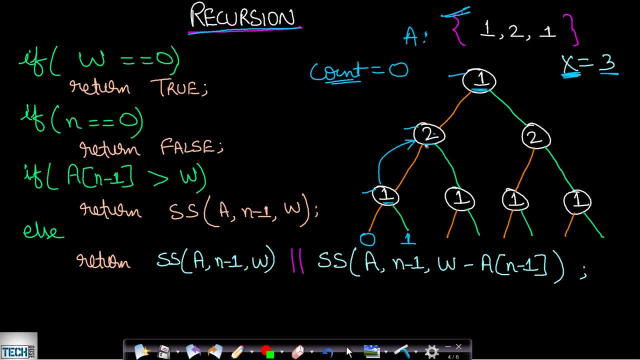 backtrack to one again from one, you backtrack to this two. Now, once you go to this two, you had already excluded this item two. Now you will try to include it. So when you include this two, then the sum value when you reach to this one will be equals to two. Now at this one, 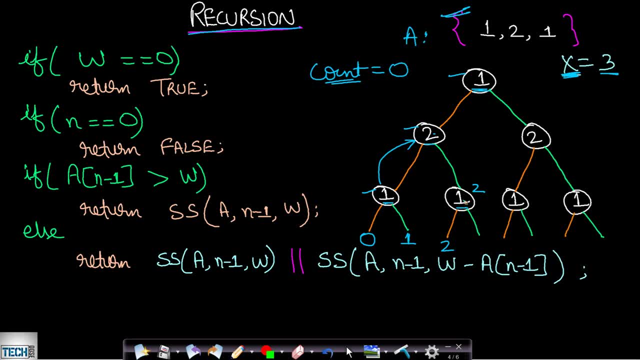 you can exclude this one to get some value equals to two, or you can include this one to get some value equals to three. So some value three is matching this x, and so you will include this one. Both those are sparsely important things to understand. You do not basically have to. 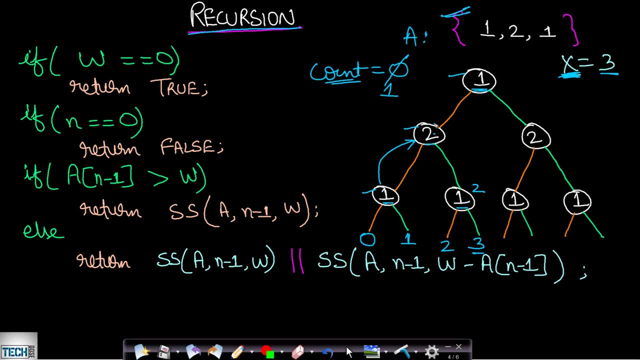 do this, So I guess I have done well by explaining the information to you. Assuming you joined me and we want to know your 들rida experience, I think that you should definitely consider subscribing to this channel. while watching this video again and again, Remember subscribe to the channel, closing the bell icon and then hit the bell. 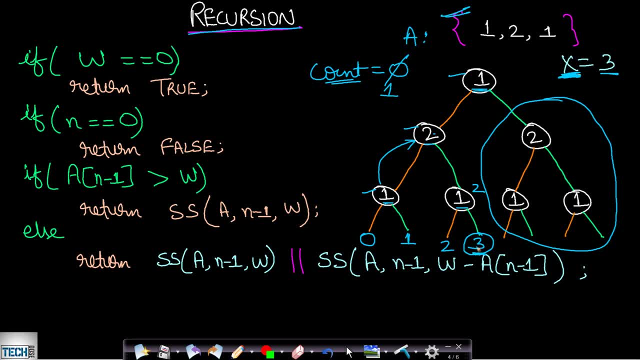 icon so you don't miss any of my updates that I upload. Now. consider this second option. In this case this happens in the domain name of the domain value, but all possible values. so we will have to keep searching the entire tree so that we will be. 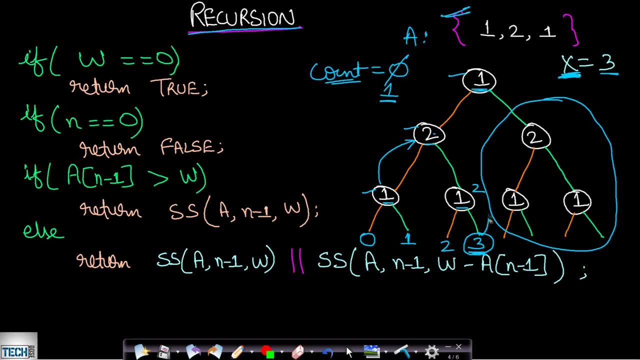 counting the exact number of subsets with the given sum. therefore, we will backtrack from here, we will backtrack again, we backtrack to one and we will search this subtree as well. okay, but in the subset sum problem we would not have done this, so we will go to two again if we include this one. 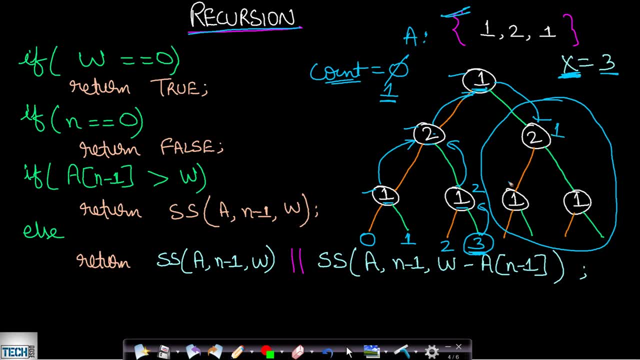 then some value here will be one. if we exclude this two, some value will be one here. if we exclude this one, some value will be one. if we include this one, some value will be two. now we will backtrack to two. again, we will include this two. if we include this two, some value will be three. 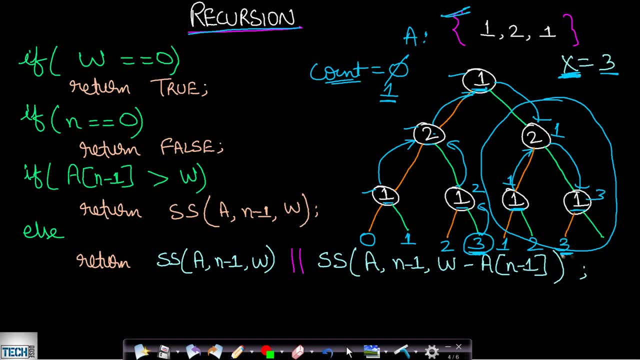 here. if we exclude this one, some value will be three, so this three is again matching and therefore this count will be incremented. so this count will be equals to two. now we will backtrack from one. we will include this one. some value will be four, so this will not be counted. now we have traversed. 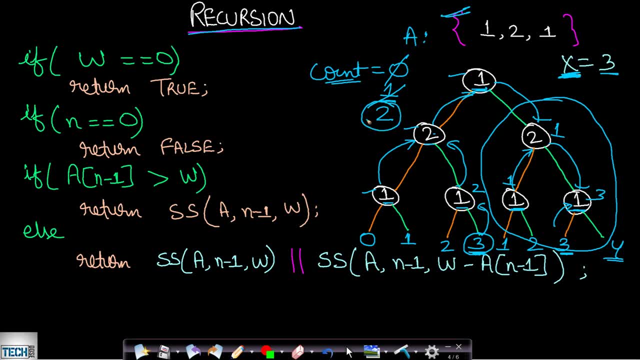 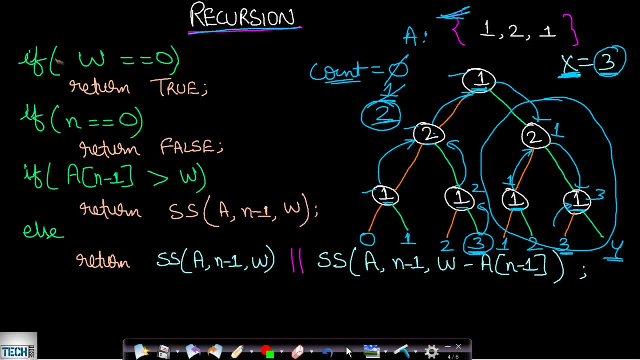 you got the understanding of how this recursion is working. now this recursion code on the left hand side is for the subset sum problem. there we were returning true if we can find a subset with the given sum. otherwise we were returning false. okay. so in each step we were doing four checks. 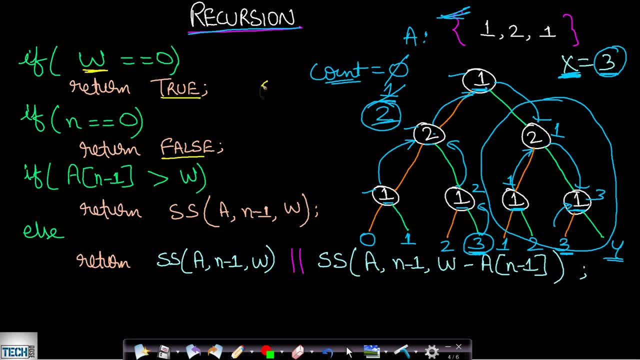 so the first check was: if our capacity of the knapsack is full- it's totally full- then obviously we have completely filled the knapsack by using a single subset and so we will be returning true. otherwise, if we have no items left and obviously the knapsack was not full, then we will be returning. 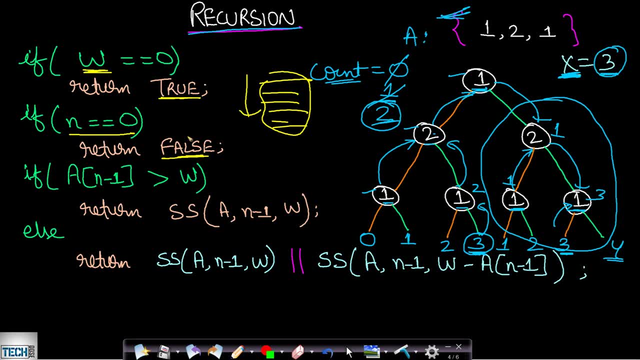 false because if all items are traversed, then we will not be having any items to include, so we will be returning. true, if we have no items left, then we will be returning. therefore, the bag can never get filled. therefore, we will be returning. false, and this was the case. 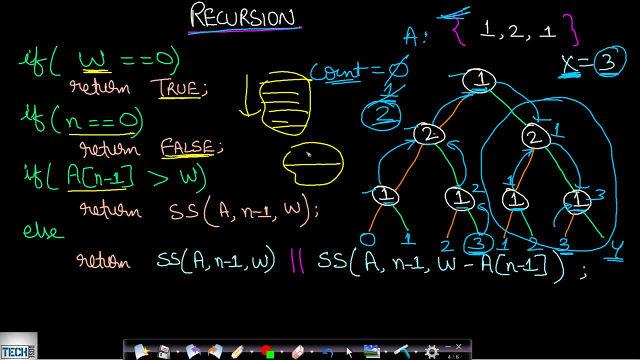 when, if you are having a bag- and this was your space left- then the single item, which is a at n minus 1, was greater than the leftover space. so this current item cannot be accommodated in the leftover space, so we will simply be skipping it and making a call to the previous item. otherwise, 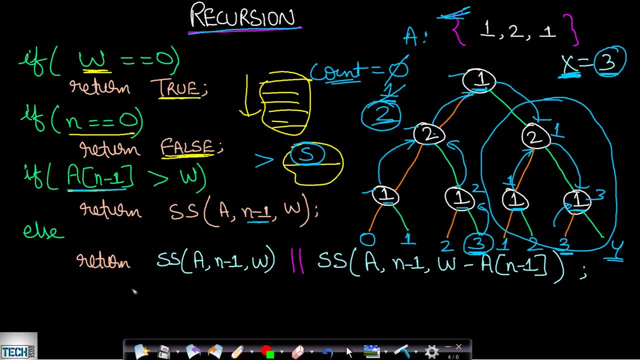 if we can accommodate an item, then, according to the choice diagram which i had shown in the subset sum problem and also in the 0: 1 knapsack problem, we will be having two choices: we can either include the item or we can exclude the item. okay, so whichever is returning true, we will. 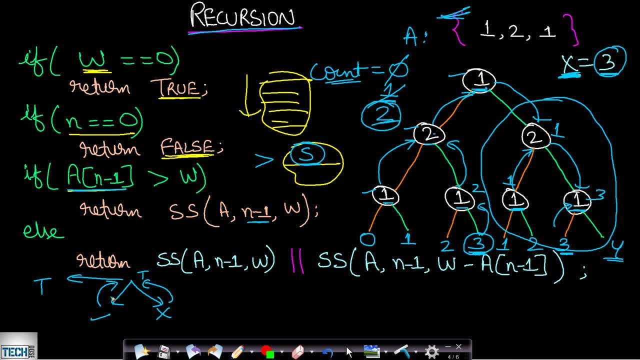 take that and we will return true as an answer. otherwise, if both of them are returning false, then we will be returning false. okay, so that is why we will be using or operator here. so this case is for x, x, x and this case is for inclusion. so if we are excluding the item, knapsack capacity will be 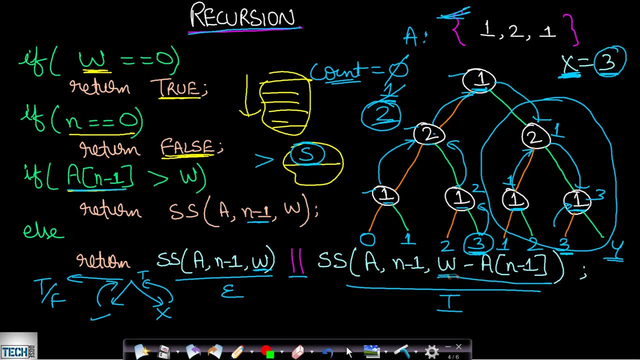 same. if we are including the item, then the knapsack capacity will decrease with the weight of the current item. so the current item is actually n, but we are taking n minus 1 because the items array this one will be starting from 0. okay, but we are actually counting from 1. i will 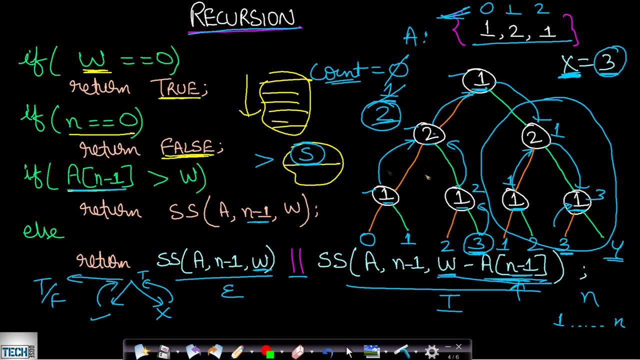 be explaining this in the dp table and i have also explained this in our previous video, so link for all those videos will be present in the description below. now, what about this problem? how do we modify this entire code in order to solve this problem, the current problem? in this case? we 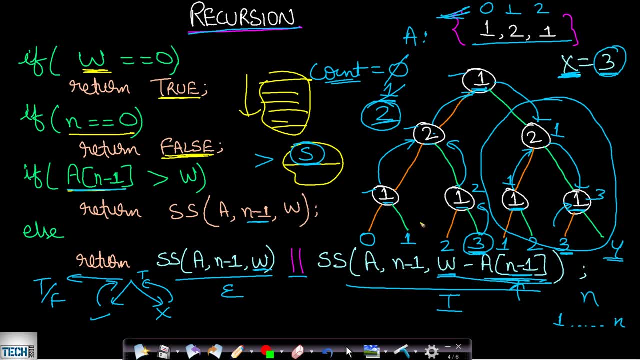 are required to count the number of subsets, and we do not just bother about returning if the given subset with the sum x is present or not. therefore, in this case, the return type will be integer, and so if we are finding a subset with the given sum equals to w, that is x. 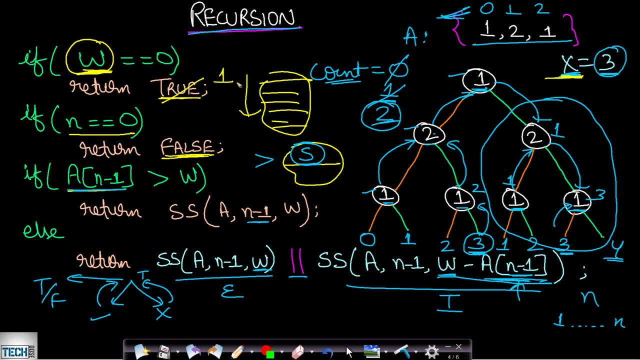 then we will return 1, saying that we have found a subset which is having sum equals to x. otherwise, if we are not able to find, then we will be returning 0. okay, this is one condition now when we are taking this- or we were basically checking for true and false conditions, but in this case 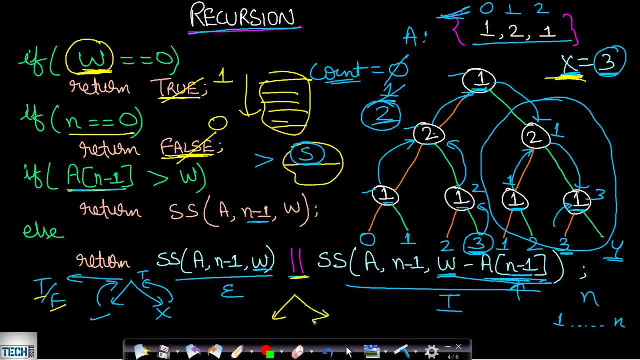 since we are counting, so we will be adding both the possibilities. let's say, on the left hand side you got a number of subsets having sum equals to x, and on the right hand side you got b number of subsets with sum equals to x. and what do i mean? 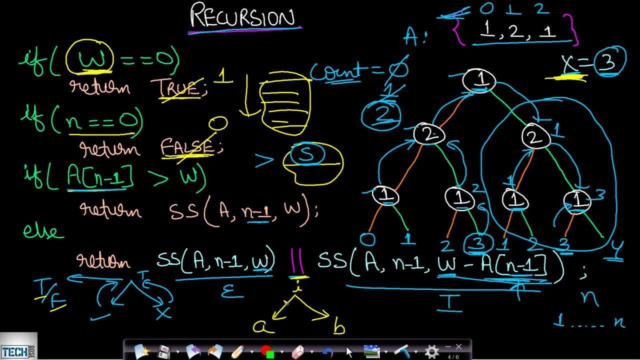 by this left and right. actually, if you are having an element i and if you are including it, then you got a number of subsets having sum equals to x, and if you exclude this item i, you are getting b number of subsets which are having sum equals to x, so the total number of subsets will be equals to. 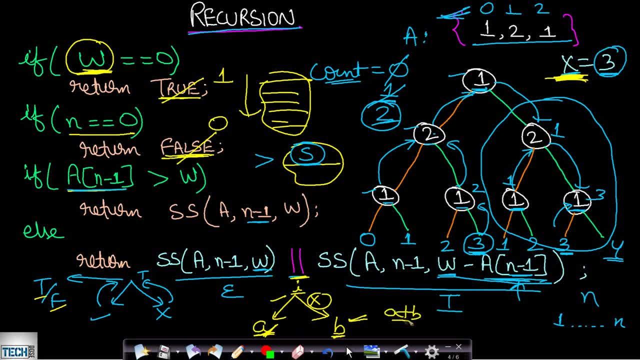 a plus b. okay, so that is why we will be replacing this or with plus, because we want to find the total number of subsets in all the conditions. whatever may be the condition, either you include it or exclude it- the sum value should be equals to x. okay, therefore, we will replace this or by plus. so this is the only change we need to. 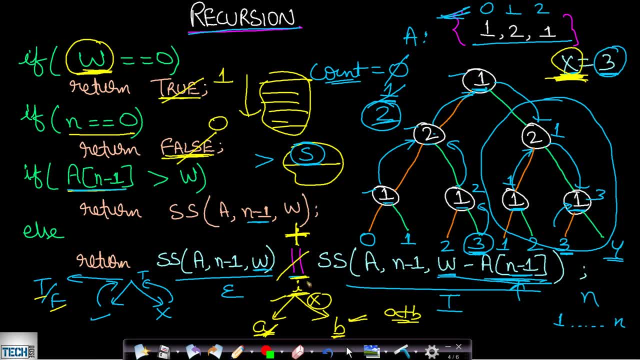 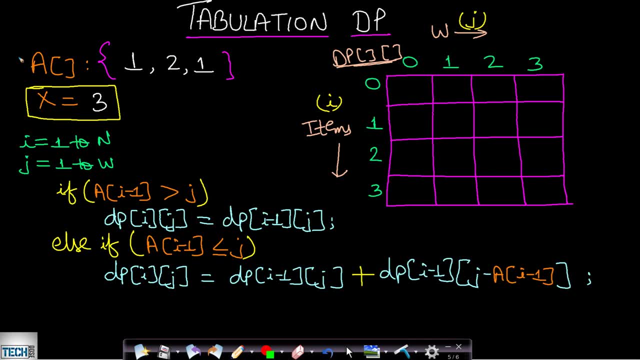 make in the subset sum problem in order to solve our current problem. so i hope you understood the recursion approach. now let us look at the tabulation dp method. now in this approach I will be taking the same example: array a and some value. x equals to three. now I have drawn the db table as I had shown in the subset sum problem, so here the rows will: 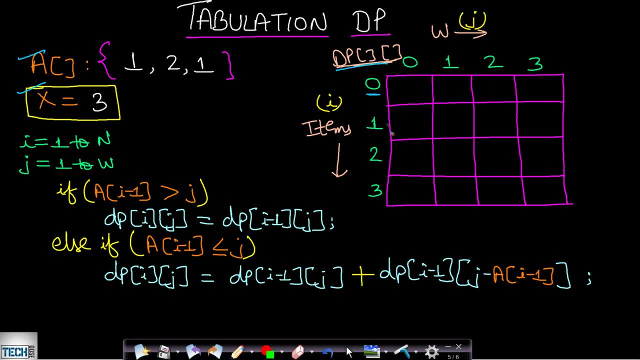 be showing the number of items, starting from number of items equals to 0 to all number of items, and our weight will be indicated by j. okay, and that is nothing but the capacity of the knapsack: 0, 1, 2, 3. this final number, 3, is actually the sum value. sum equals to x. okay, and this last cell will be giving. 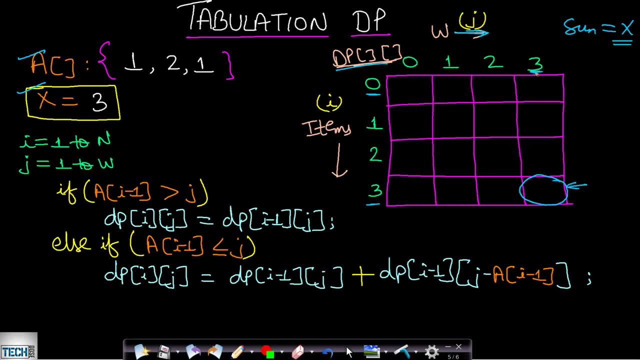 the total number of subsets having some value equals to x. given this array and this given sum, okay, now let us fill this db table now. in this case, this first column is indicating that we are having no capacity in the bag. that is, our sum value is equals to zero. so how do you form in? 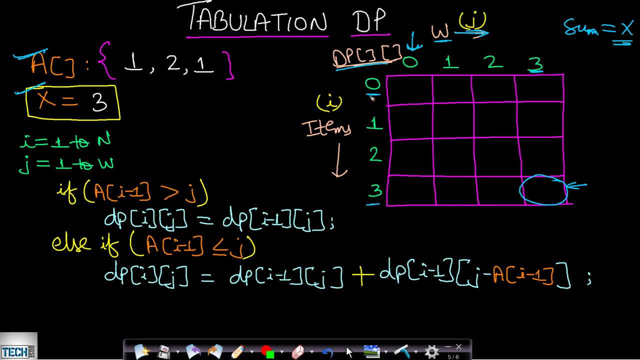 how many ways can you form some value equals to zero? now, it doesn't depend on the number of items, how many you have in your array a. you can just take an empty subset and you can say that the sum of this subset is equals to zero. so there is only one possible subset, which is this empty subset. 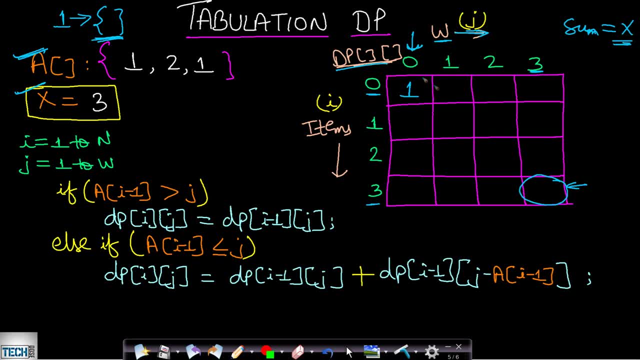 therefore, there will always be one possible subset having some value equals to x if x value is equals to zero. therefore, we will be filling this first column with value one, because it will always be possible to find the sum value of this column in the array a, and in the array a you can just. 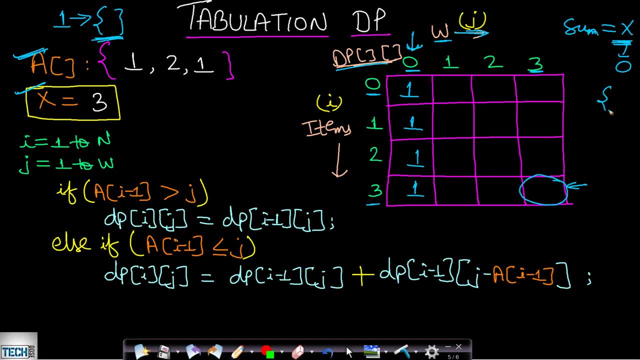 equals to zero and there will always be only a unique subset, which is this empty subset. now, what about this first row in the first row, leaving this one? if you are having no items and if the sum value which you require to find is greater than zero, then obviously you cannot. 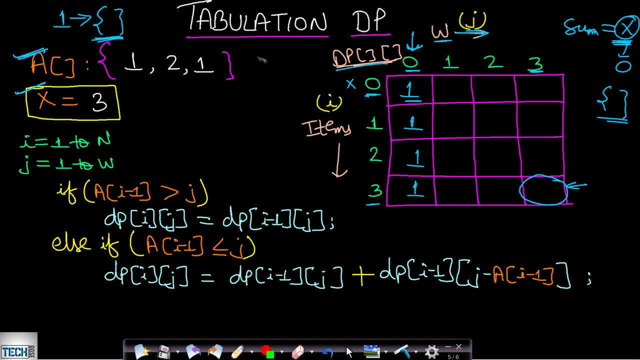 take any item, and so you cannot form any sum because you are having just an empty subset. if you have no items, then obviously your array a will be equals to an empty array, and if you are having empty array, then you cannot form any sum other than value zero. 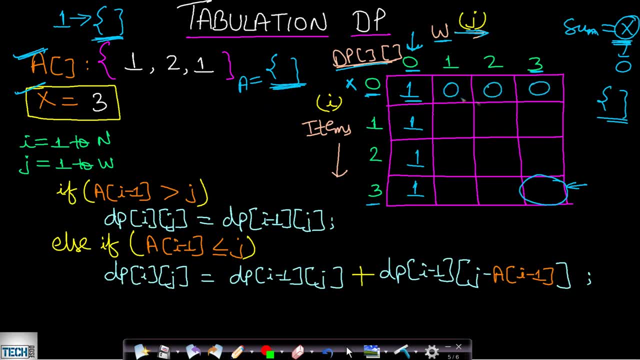 and therefore all these sums cannot be formed, and so we will just be writing zero number of subsets there. now we will start filling from this part, first column and first row. okay, so we will be taking two loops in order to iterate through all the cells. i will be trading through the items. 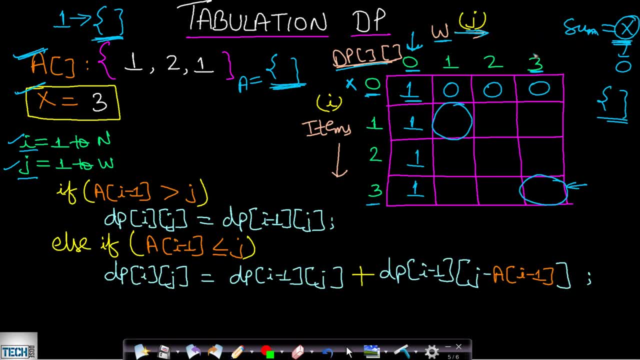 and j will be taking the items, and j will be taking the items and j will be taking the items, be iterating through this uh, knapsack bag, which is nothing but this w, that is the sum value. now, in the first row, we will be pointing to this one now, according to these two conditions, this one 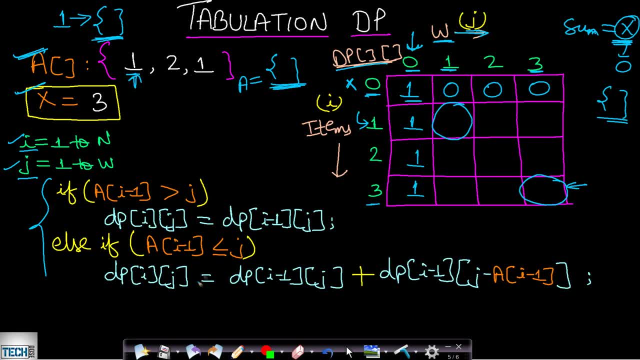 is actually greater than equals to this sum value. so dp at ij will be equals to. this is exclusion part. okay, so either we can exclude this item or include this item, because this item weight is actually less than equals to the capacity of the bag, which is one. so we can either include it or 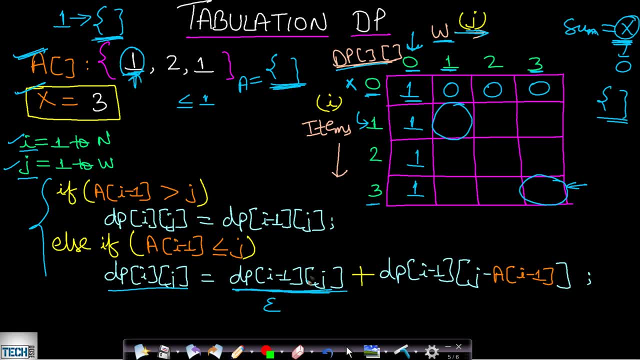 exclude it. so if we exclude this, then the number of subsets with given some x will be equals to the number of subsets with given some x having one less number of elements. okay, so since our sum value is equals to one, and if we decrease one item, then we will go to the previous item. 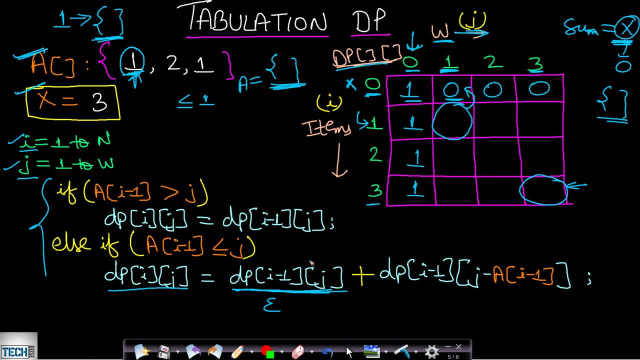 which is zero number of items. so we will have value zero here and we will be adding if we include this item. if we include this item, then how many subsets do we have actually? so we will be going to the previous item, since we have included this item. 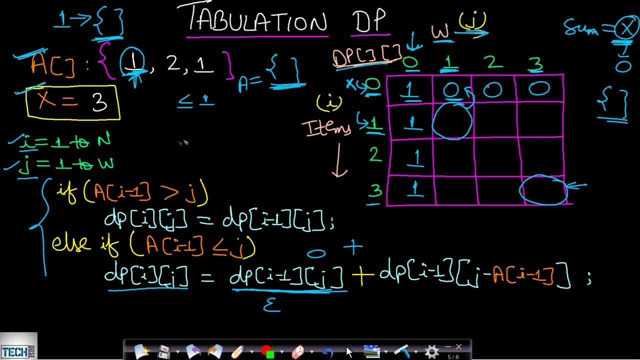 and then the capacity of the bag will be decreasing and current capacity is one, the current value, which is included, is one, so the remaining capacity will be zero. so we will be going one item less, that is, we will be going to i minus one and at capacity zero, that is, dp at i. 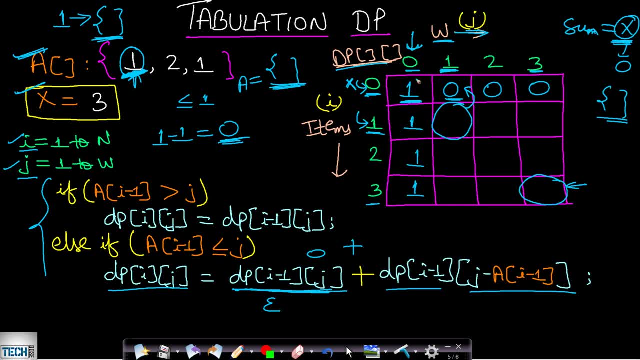 minus one, j minus a at i minus one, so that value is equals to one. so this will be one. so zero plus one will be equals to one. therefore, we will be filling one here. okay, i hope you are understanding how i am filling this now. these are the two cases according to the choice diagram. this is the 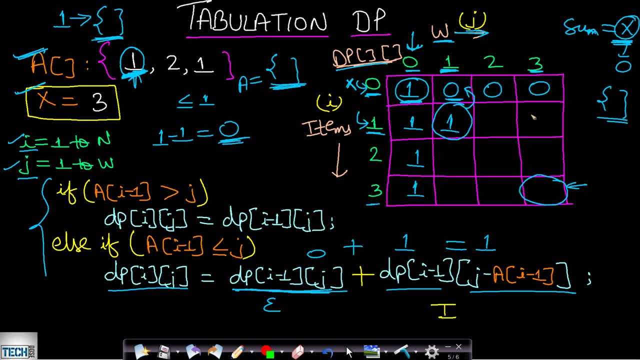 inclusion case. now we will fill similarly the rest of the cells. now for this cell here, we will either be including it or excluding it, because this weight value here is less than equals to this. now, if we exclude this, then some value will be, this one zero, and if we include this, then some. 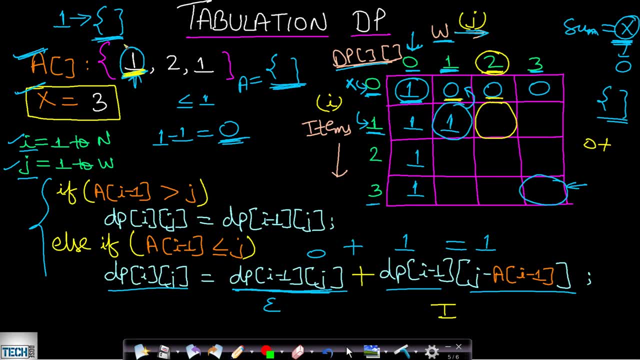 value will be this one, because the weight of this is one, and if we include this, since the capacity is two here, and if we include this weight one, then the left over capacity will be one, with one item less. so this zero plus zero will come out to be zero. so therefore this will be zero and similarly, 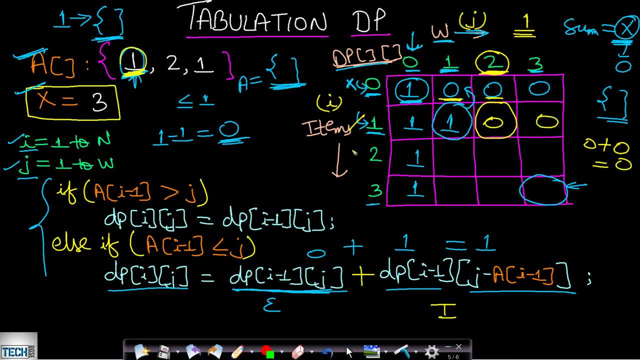 this will be zero. now we have filled for single item. now let's point to two items. so if we are having two items- this one and two both- we are having both, both the items. now if the sum value is one, then how many number of subsets can we form with sum equals to one? 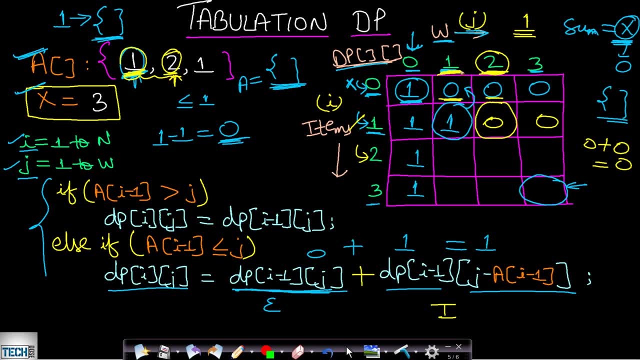 so this value 2 is actually greater than the knapsack capacity, which is one here. okay, so that is why here we cannot accommodate this. we will have just a single choice. so we will be basically hitting this if condition, and so we will just be, uh, having one choice of a. 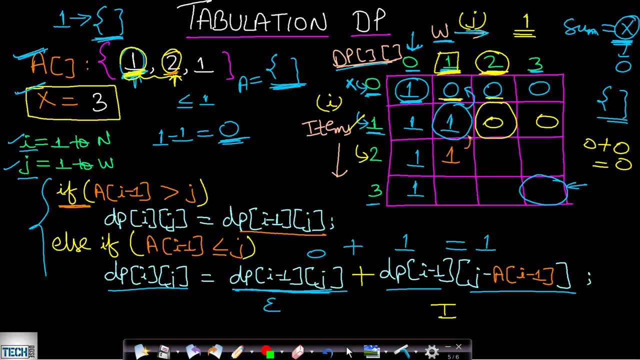 sub set. okay, so now we will have two choices: which is the item weight, which is the top value, which is the item weight, which is the exclusion case. we will simply be copying the top value because we cannot include this item. therefore, we will be having one items less and whatever is the 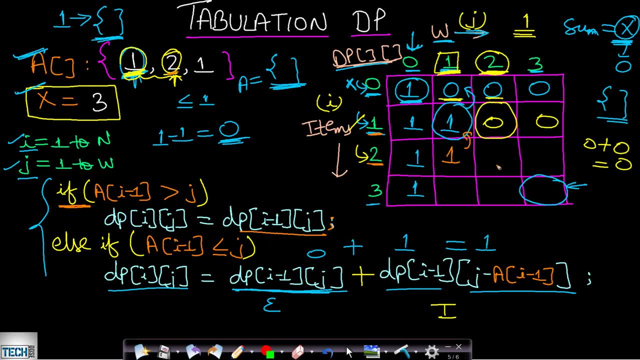 maximum number of subsets formed by one item less. that we will just be copying. okay, this i have already explained in the subset sum problem. now we will move on to the next cell, this one. so here the include. if we exclude, the sum value will be this: zero plus, if we include this item, weight two then 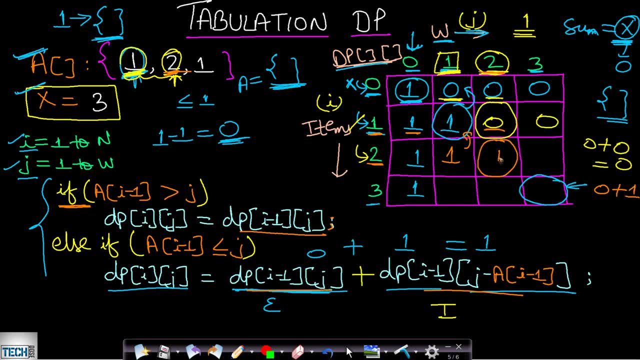 sum value will be this one, so zero plus one will be one, and similarly, for this one it will come out to be one. now let us fill this last row. so for this last row, it indicates that we have all the three items. now this last one is having value one. so we will have two choices: we can exclude or 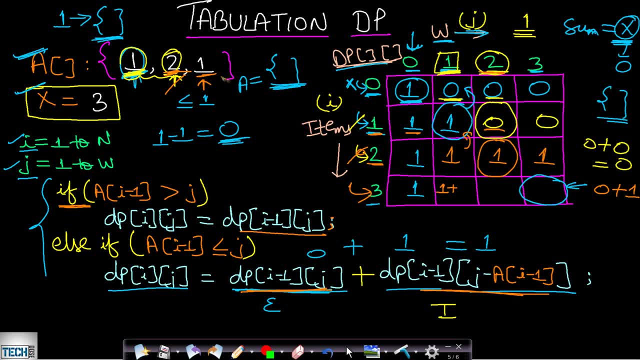 include. if we exclude, the sum value will be one, and if we include, then the sum value will be this one. so one plus one will be two. similarly, for this one it will be two, and for this one it will be two. now, this is the total number of subsets with the given sum value, x, which is three in this case. 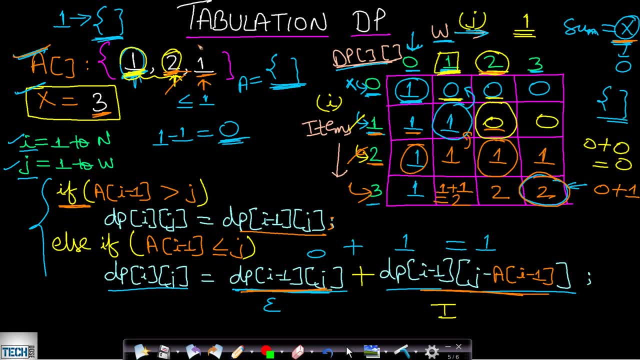 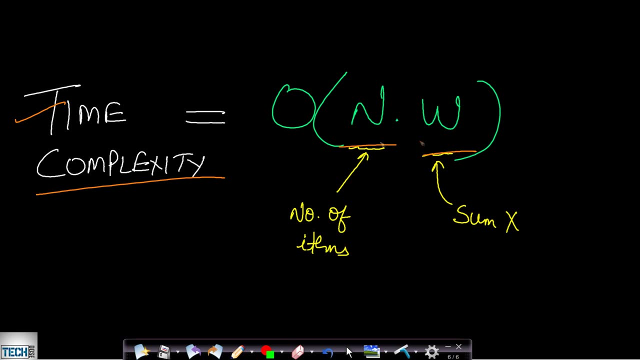 which can be formed from our given array, that is, our given set. okay, so i hope you understood how to solve this problem very, very simply. if you already know the subset sum problem, then this will be a just a cakewalk. now, what is the time? complexity? it is equals to order of n into w by using the